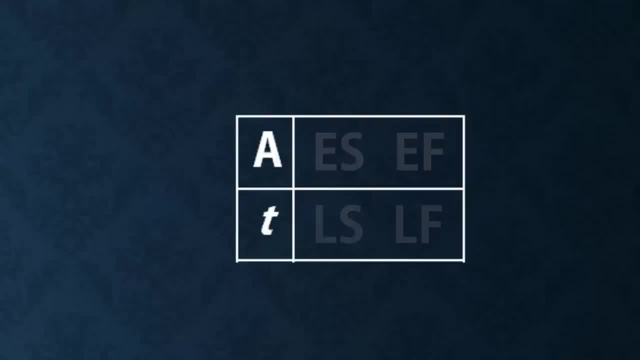 as you will find in Quantitative Methods for Business by Anderson, Sweeney and Williams. A- here is the activity being described and T represents the expected activity duration or time. ES is the earliest time the activity can start. EF is the earliest finish time. 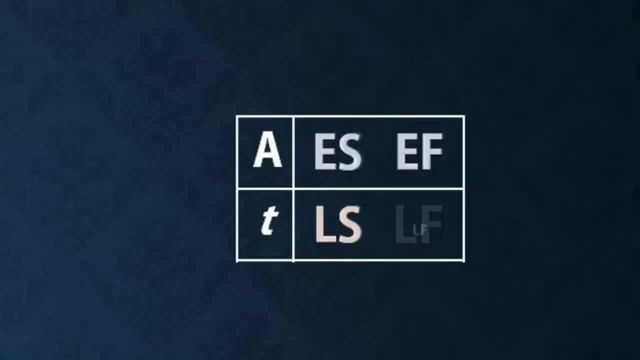 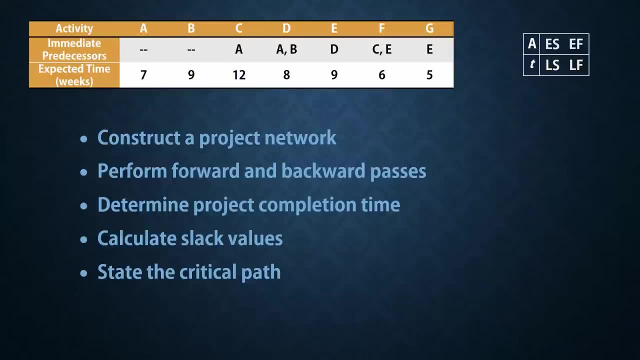 LS is the latest start time And LF is the latest finish time, without extending the minimum completion time of the project. I usually like to start with a sketch to make it easier when drawing the full network. Activities A and B have no predecessors, so they can begin or start. 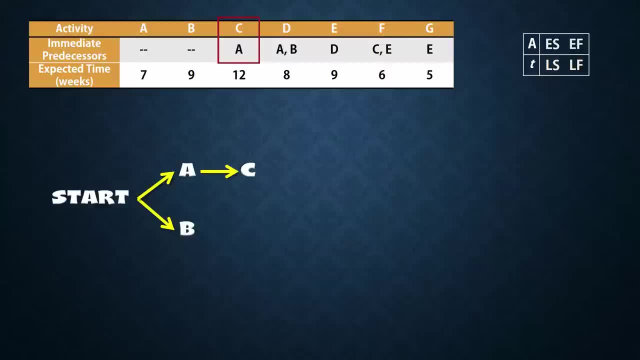 Activity C needs A to be completed before it can start, D needs both A and B completed, E needs D, F needs C and E, And G depends on E. Since F and G have no successors, they go to finish, But it will take some time. So here is the network with the activity nodes. 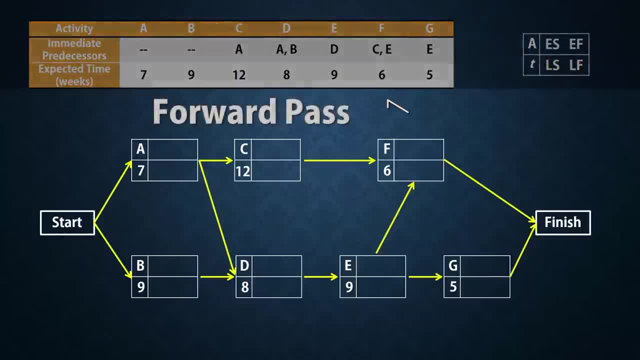 displaying the letters and times. So let's do the forward pass…. Activity A has no predecessors, so its earliest start time will be zero or right away. Since it has 7 weeks to be completed, its earliest finish time will be 0 plus 7, which gives 7.. 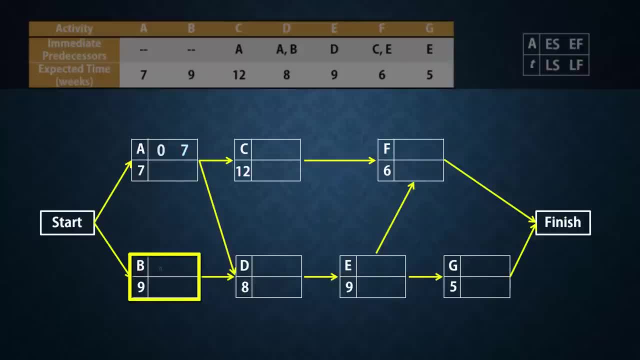 Activity B also has an earlier start time of 0 and with an activity time of 9, it will have an earliest finish time of 9.. Activity C needs C to complete at an earlier start time of 9.. Now C needs A to be completed before it can start, Since the earliest finish time for A is 7,. 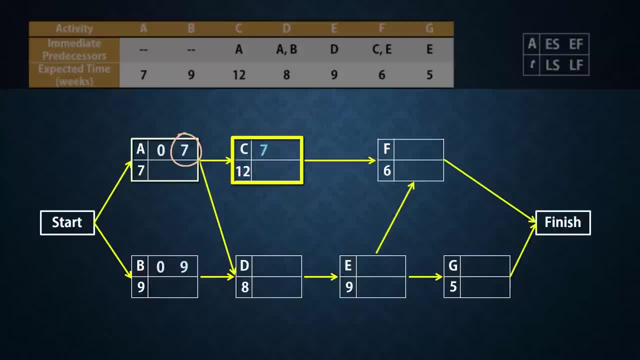 then the earliest time C can start is 7.. And with an activity time of 12 weeks, C will have an earliest finish time of 12 plus 7, which gives 19.. D, on the other hand, needs A and B to finish before it can start Since the earliest finish. 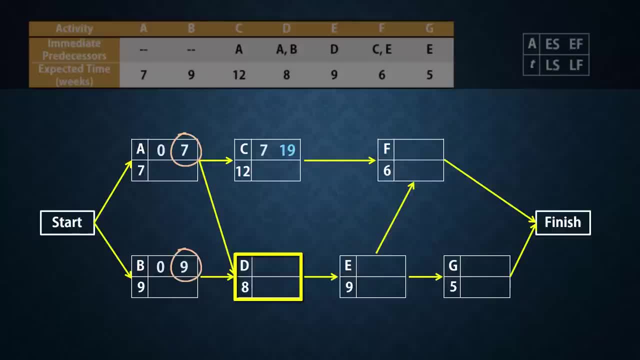 time for A and B are 7 and 9 respectively, and D needs both of them to finish in order to start, then the earliest time D can start is 9.. In other words, the highest of the earliest finish times preceding an activity will be the activity's earliest start time. So D finishes at 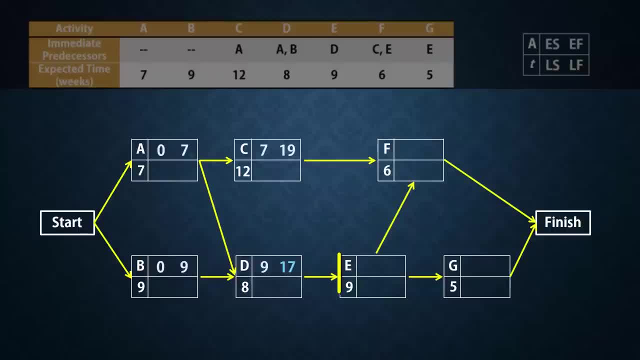 8 plus 9, which gives 17.. E here has only one predecessor D, and so can start at 17 and finish earliest at 27.. F has predecessors C and E. Since the higher earliest finish time is 26,, F can start earliest at 26 and finish at 32.. G also can start earliest at 26,. 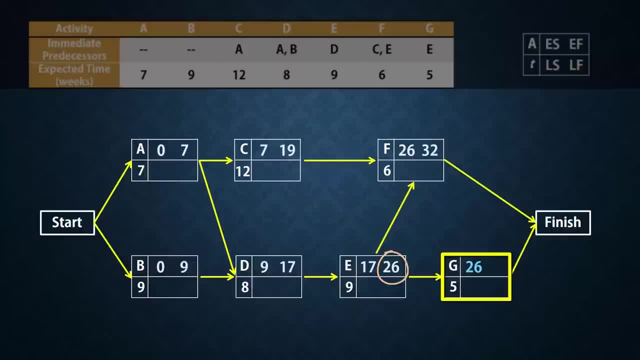 since it has only one predecessor, E and G can finish earliest at 26 plus 5, which gives 31.. Note here that although G is the last letter, it doesn't have the highest earliest finish time, 32, so we say that the project's completion time is 32 weeks. 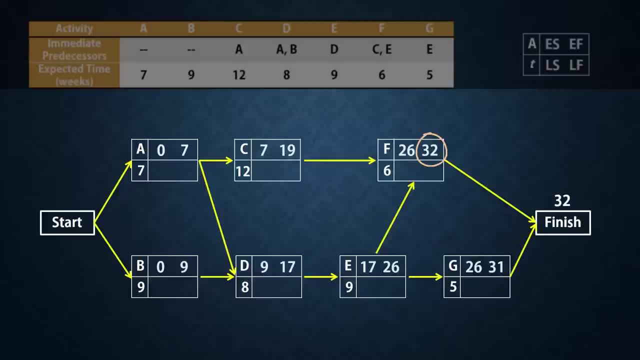 In essence, the project's completion time is the highest of the earliest finish times at the finish node. Now let's do the backward pass. Since the project's completion time is 32 weeks, the latest finish times for the activities at the finish node F and G has to be 32.. 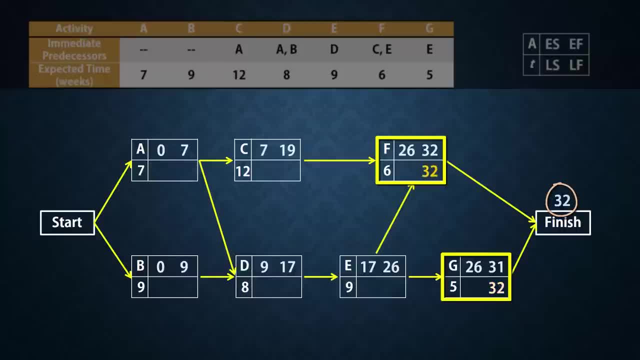 That is, F and G, cannot be completed in longer than 32 weeks. Next, we obtain the latest start times by subtracting the activity times from the latest finish times. For G, the latest start time will be 32 minus 5 to give 27.. 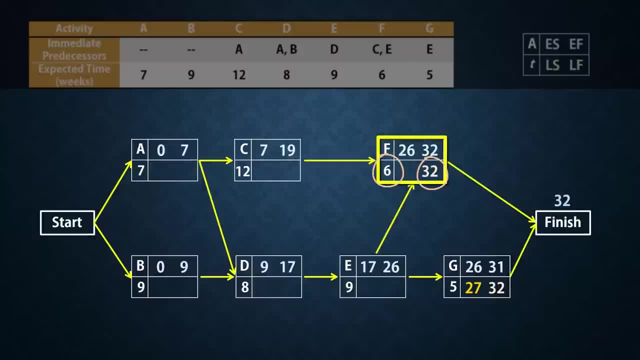 For F, the latest start time will be 32 minus 6, and that gives 26.. Now E has two successors, F and G. The latest start times are 26 and 27.. As a result, the latest time E has to finish has to be 26 in order for F to start. 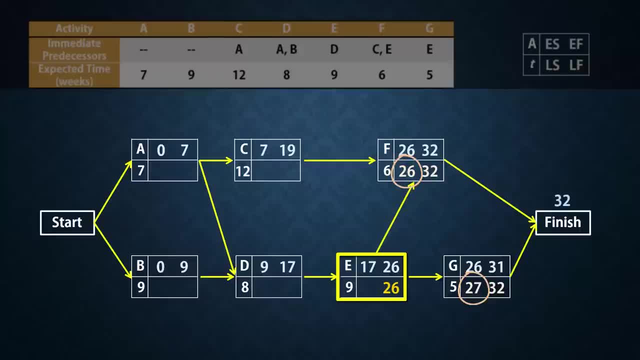 In essence, when doing backward pass, the latest finish time of an activity must be the minimum of the latest start times of its successors. Thus, the latest start time for E will be 26 minus 9, which gives 17.. Now D has only one successor, E, So the latest finish time for D will be the latest start. 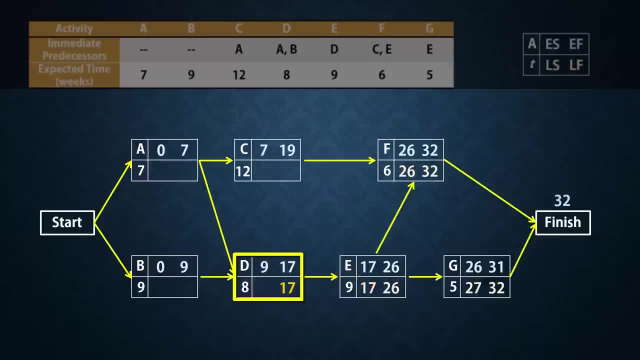 for E, which is 17.. And the latest start time will be 17 minus 8, which gives 9 for D Activity. C has one successor F. Therefore the latest finish will be 26 for C and latest start will be 14.. A has two successors: C and D. The minimum of their latest starts is 9..